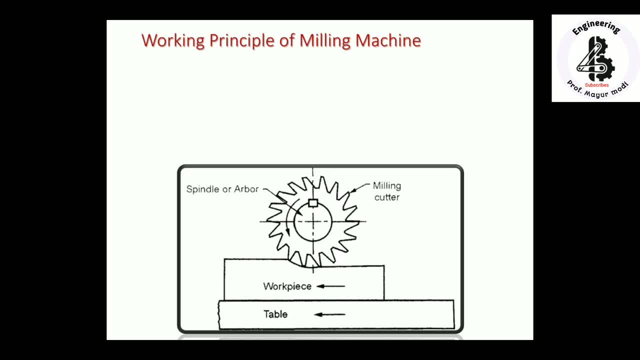 spindle and workpiece is directly mounted onto the table with the help of some of the clamping device, or you can also use the some of the clamping vise to fix the workpiece and carried out the different machining operations onto the milling machines. so just you can say the metal removal. 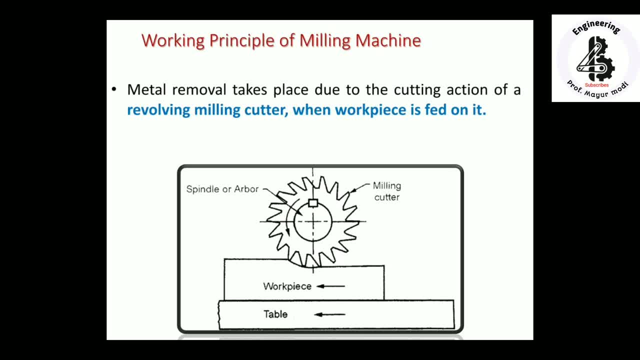 take place due to the cutting action of a revolving milling cutters when the workpiece is fit on it. so, according to your required shape and size of your job, you can use the different size and types of the cutters. so cutter is hauled into a spindle or arbor. operation is performing. 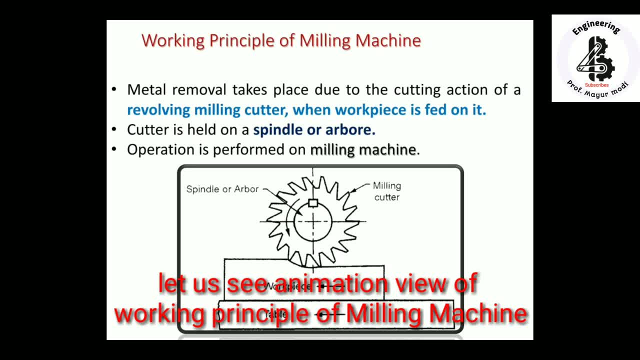 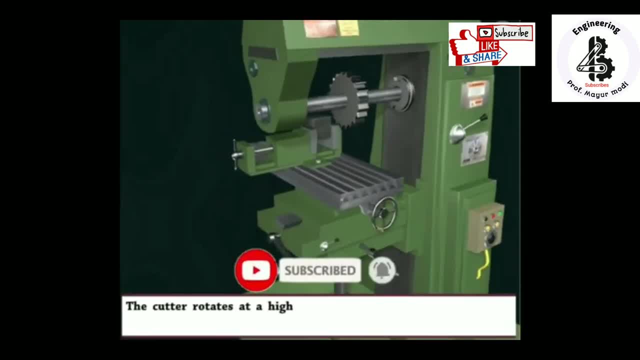 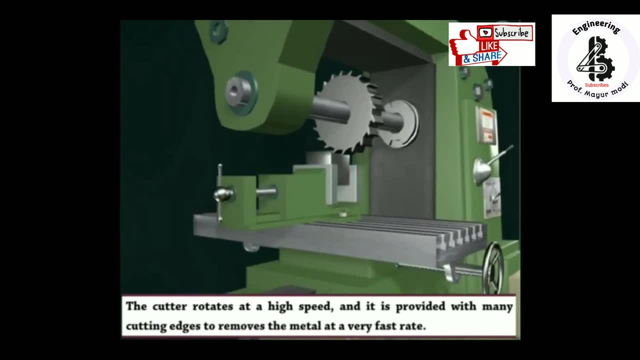 on a milling machine. so that would be called as a working principle of a milling machine. so it is pretty cool. At the end of the day, a milling machine is a better tool than a wood cutter. if you are using other types of workpieces like this one as a milling machine, you can. 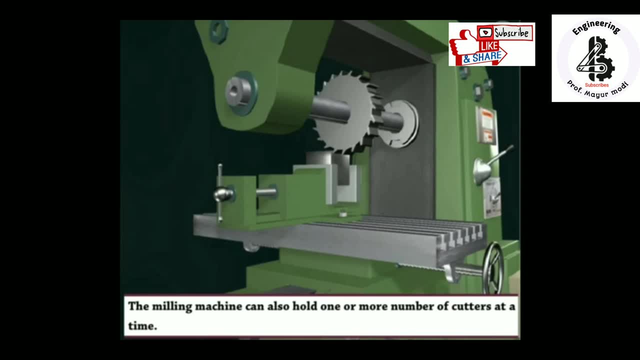 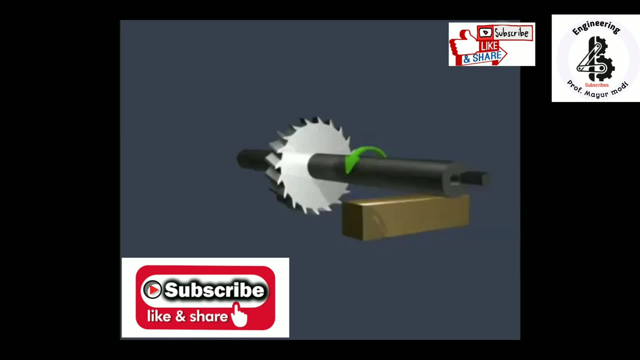 go ahead and get a good old milling machine. this one is a lot easier to use and the difference between the two is that the milling machine is more than a good old milling machine. you can use the same milling machine for a lot of different workpieces and tools and they 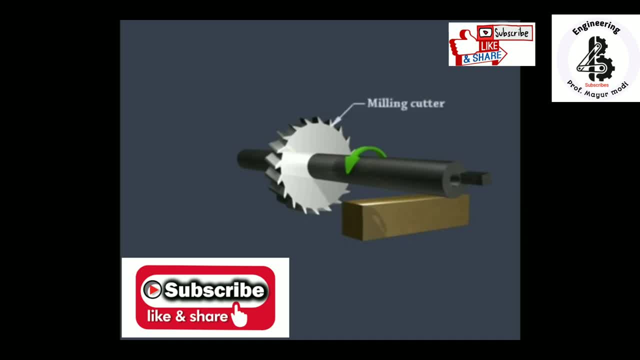 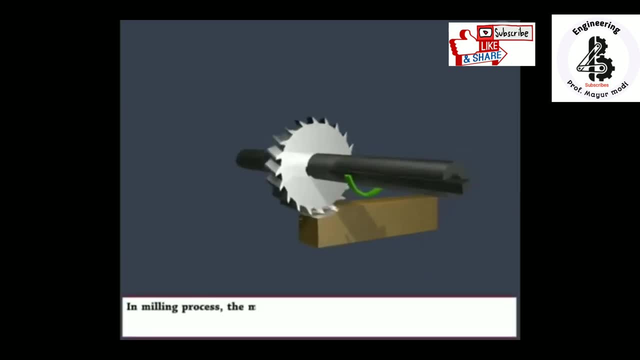 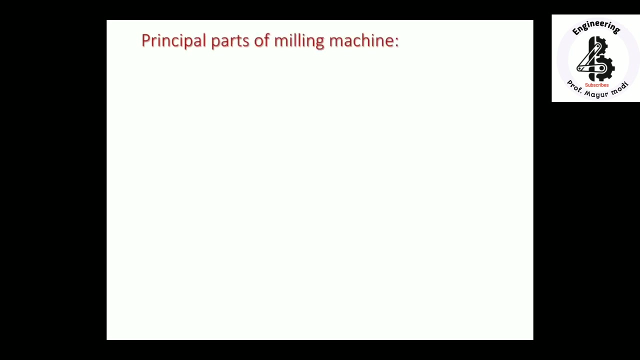 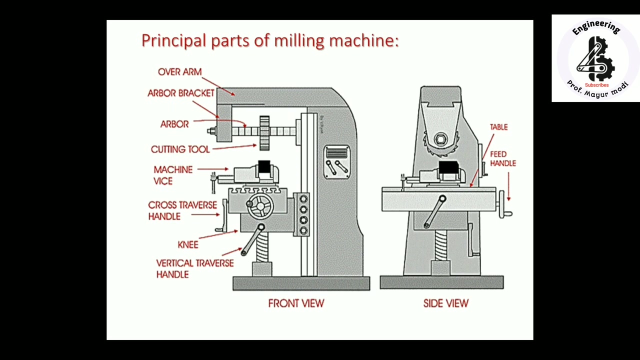 all have the same workpieces, which are not Isaac, and they all have the same milling machine, of course. so let us start with the principal parts of a milling machines. so just you can see over here there are so many components- is being used for easily positioning of the tool and work piece. 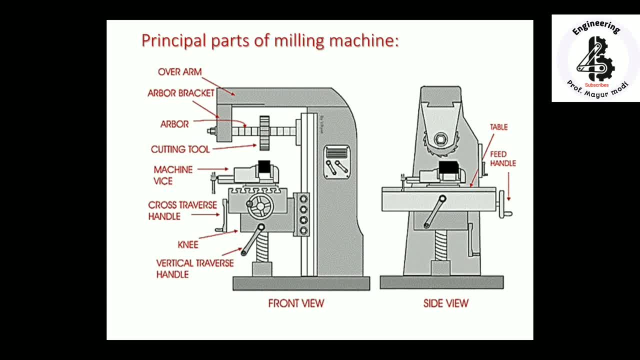 for the performing of a different positions. so here it will be the two views of a milling machines. first one is the front view and a side view, if you can see the milling machines so generally, starting with the base, then the column over arm arbor bracket, so that will be contained. 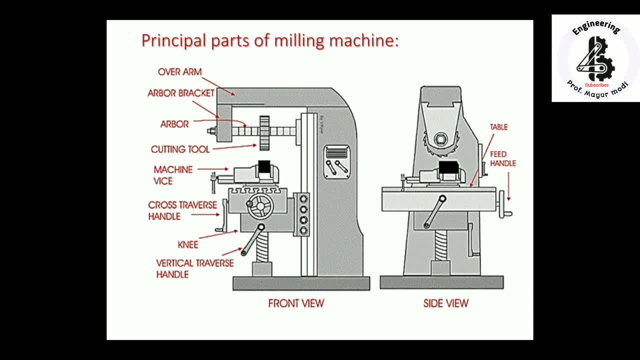 with the arbor, so on arbor cutting tools, and with the base that will be the vertical transverse handle for the movement knee cross traverse handle, then the machine wise to holding the work piece. there are so many components so you can easily controlling the feed speed. 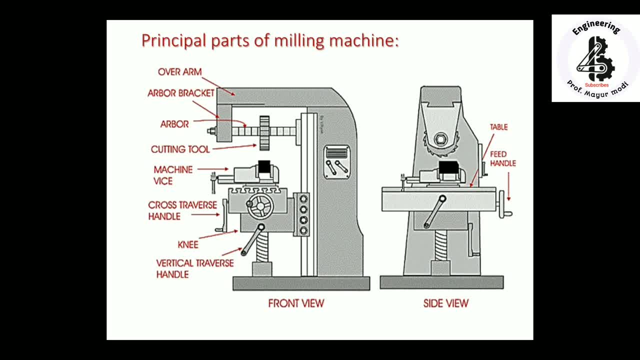 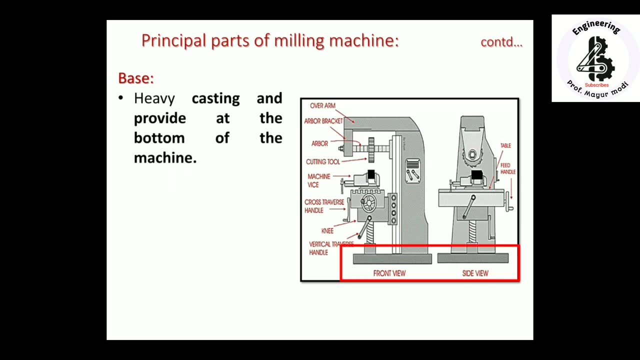 laptop card and you can also visualize or observe the how the cutting tools are used so that you can easily control the feed speed. laptop card and you can also visualize or observe the how the cutting tools are used. so it is circuit just on the vertical meditation and also there are so many amount of the 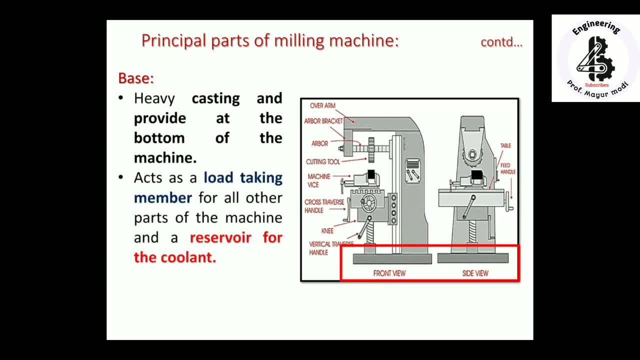 Darrenches design tools are so that you can easily control the feed speed, both alive and dead. that's basically. it's only how to do the kind of work as it has to be해, you can see, and also depending upon the milling tisi to make it the most. 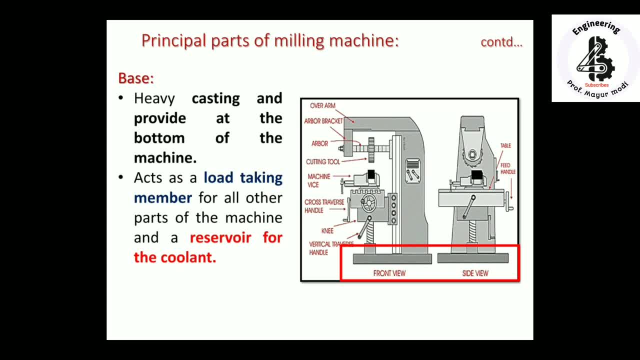 they are also find it is because they see this we still know by your own puncture mnemonics also. coolant will be transferring from the base to your cutting area and once again that will be collected onto the reservoirs. you can use the different filters and once again that will be the repeated 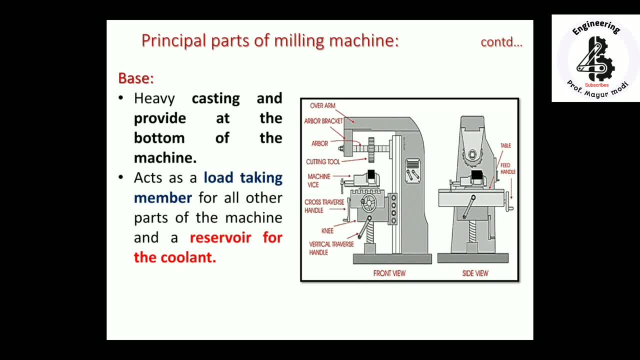 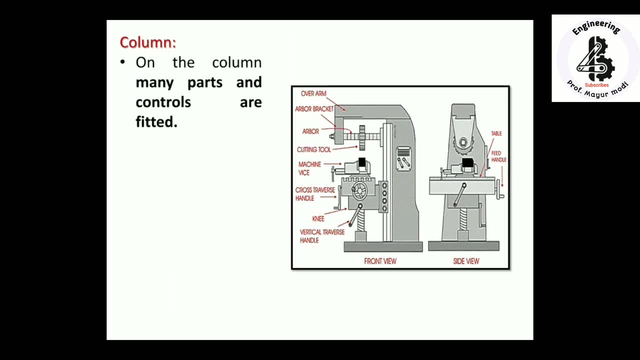 motions of the that cutting fluids. so column of the machine is secured to the base now the second one column. so that will be the many parts and the controls are fitted with the columns so you can easily controlling the machines during the different kind of operations with the different 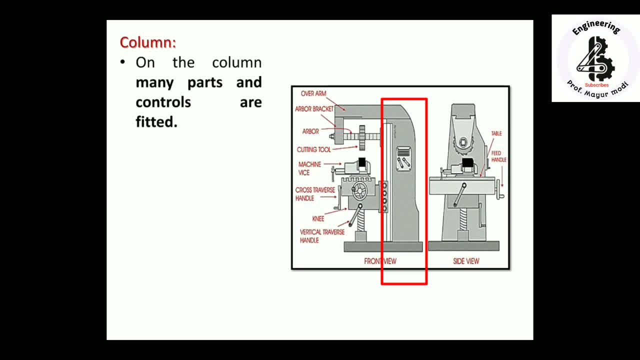 kind of cutters onto the different kind of workpiece material. then the vertical parallel guideways are provided on a front face of the column in which knee slides up and down, so you can easily adjusting the height of the job with respect to your cutting area. and once again that 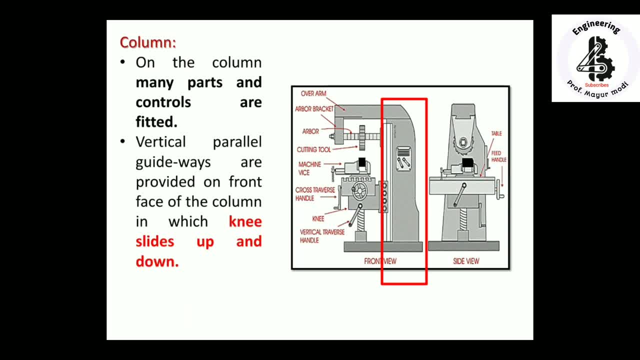 cutter positions and you can performing the different milling operations. so, on the top of the column, over arm is being supported. so with the overarms it will be the arbor brackets, arbors and different cutting tools is being mounted onto the arbors. so that will be the making a bridge between 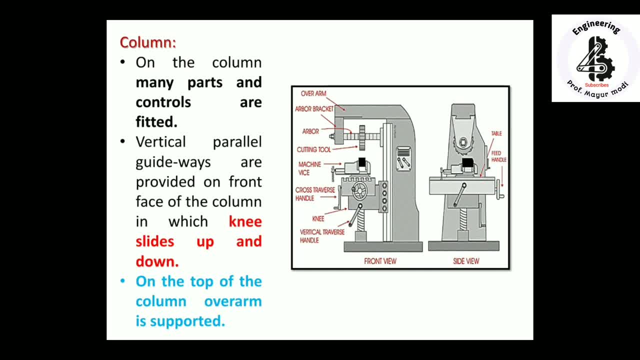 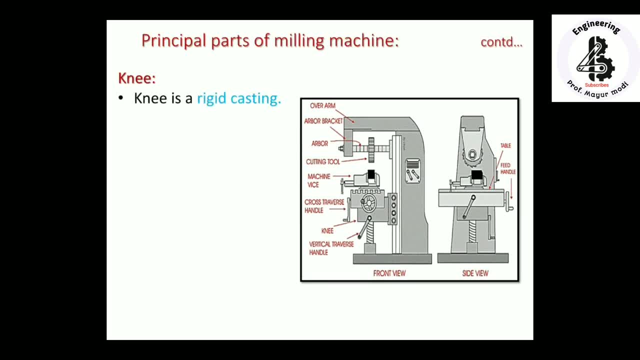 the base and the over arm and that will be having a heavy member, so that would be also resist the so many stocking loads. then knee, that will be the very important member and that will be also made with the rigid casting materials. just you can see over here with the movement of the knee, the table height or you can. 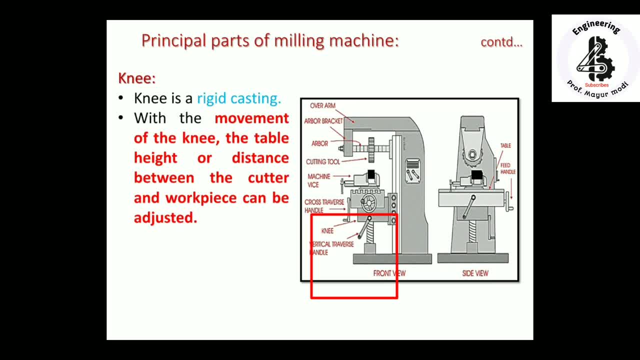 say, distance between the cutter and workpiece can be easily adjusted. that will be. you can also use by the manually, so by operating the screw jack with the help of the hand wheel, or you can say power feed mechanism is being used. so that will be the very important member and that will be also made. 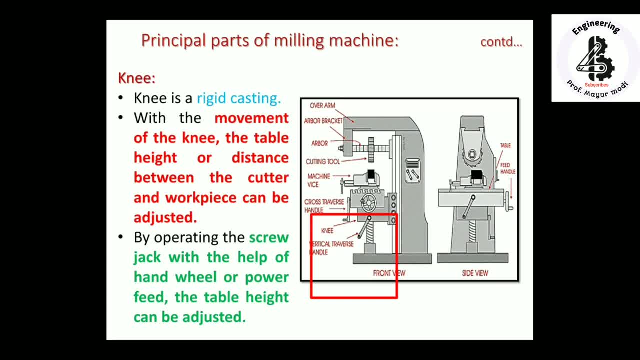 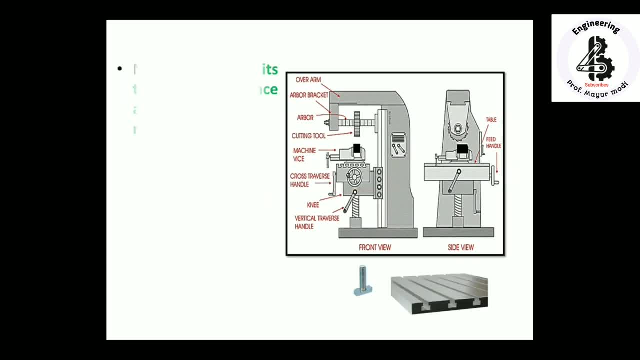 with the help of the saw and donated to the tableman and also the board with the Hit board and longer, which is it to adjust the table height can be used and that should be according to the requirement of the performing the operations. then table That will be made of the CI- you can say cast iron- with its top surface accurately machines, because that will be the area when actually the work piece is being. 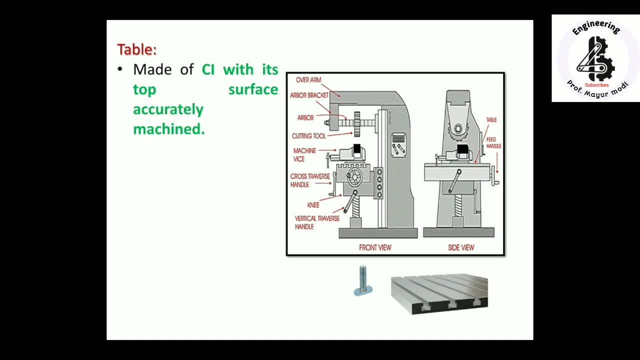 fixed on to the table. either it will be direct or you can also use with the help of machine to be able to adjust back machine-wise So to accommodate the clamping bolts for fixing the workpiece. the top surface of the table carries the longitudinal T-slots according to the figure. 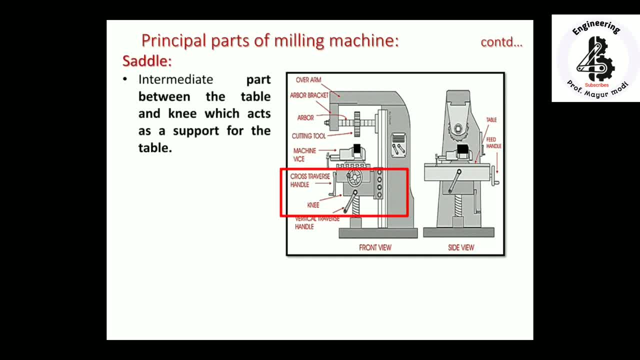 Then Saddle- important part that will be the intermediate part between the table and the knee, which act as a support for the table And to provide the cross fit to the table, the saddle can be adjusted cross-wise, along with the guideways provided onto the top of the knee. 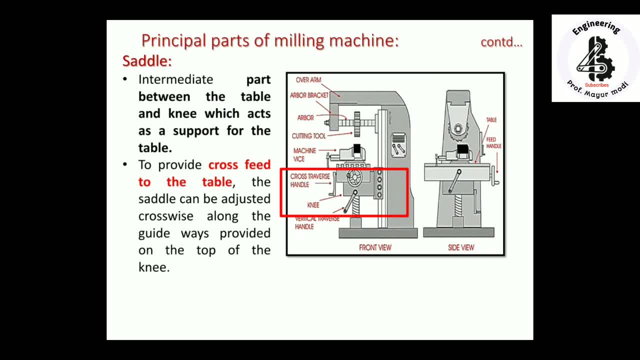 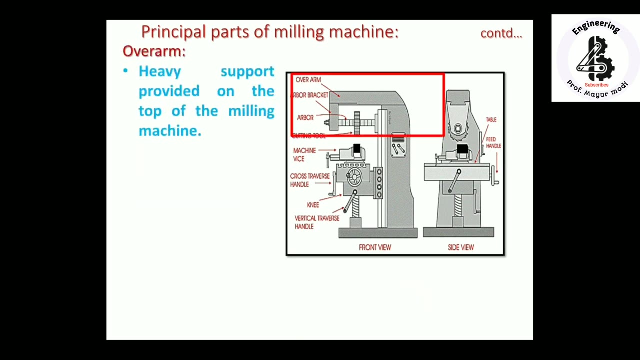 So you can easily positioning your cutter positions with respect to your required machining surface. So the horizontal guideways are provided at the top of the saddle, along with the table, can be moved into the longitudinal directions So you can easily positioning Overarm. that will be the important part of a milling machine. 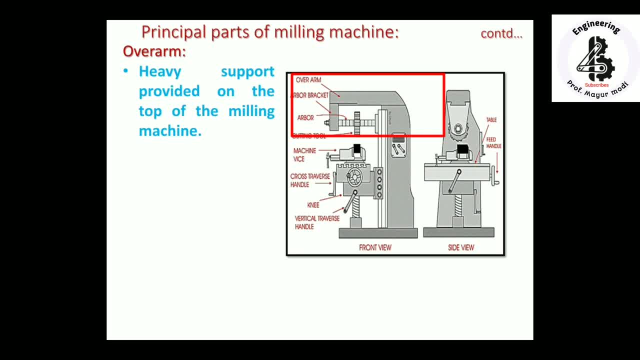 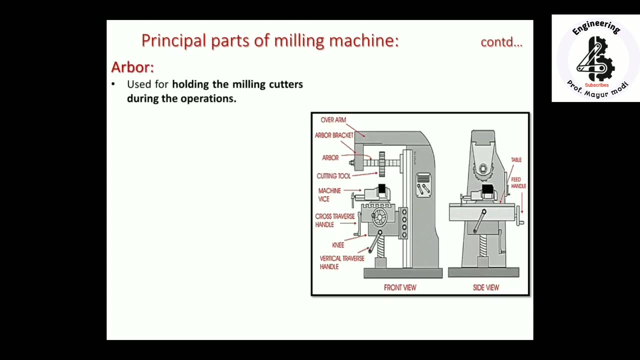 So heavy support provided on the top of the machine To support the projecting arbor. it can slide horizontally forward and backward and adjusted at the required positions Arbor so that will be used for holding the milling cutters during the operations Overarm. that will be the important part of a milling machine. 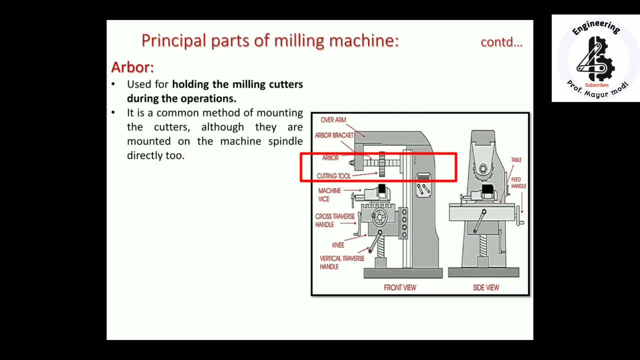 And it is common method of mounting the cutters, although they are mounted onto the machine spindle directly too. Or you can say the arbors are mainly two types of standard arbors and stub arbors. So according to my requirements, both the arbors are being used. 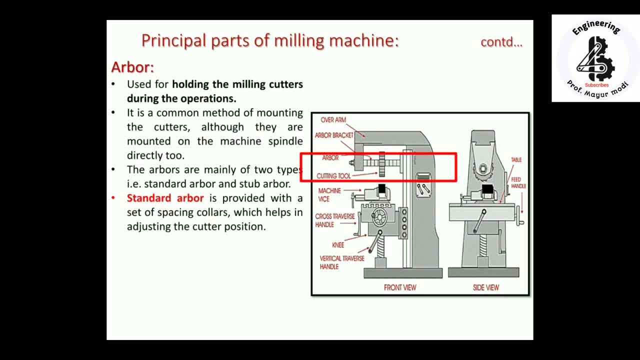 For the standard arbors it is provided with the set of the spacing collars. So collars is being used for separate out the different kind of milling cutters. So with this help in adjusting the cutter positions. the slots are provided onto the 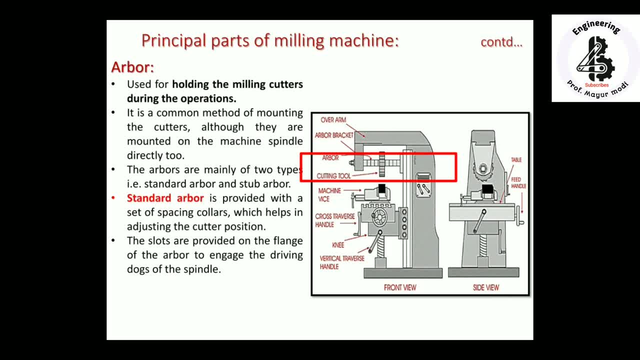 flange of the arbor to engage the driving docks of the spindles, Then the second arbor that will be the stub arbors are mainly used to hold the face and the side milling cutters which do not be need in a large overhang. 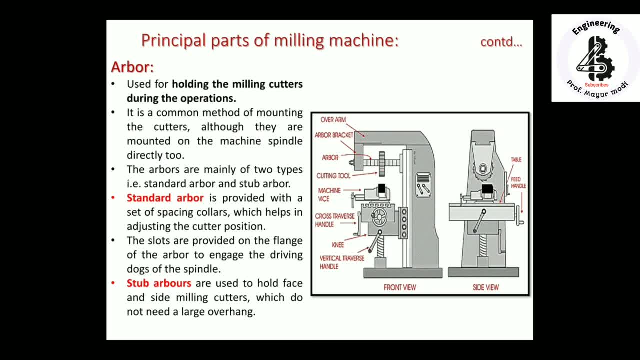 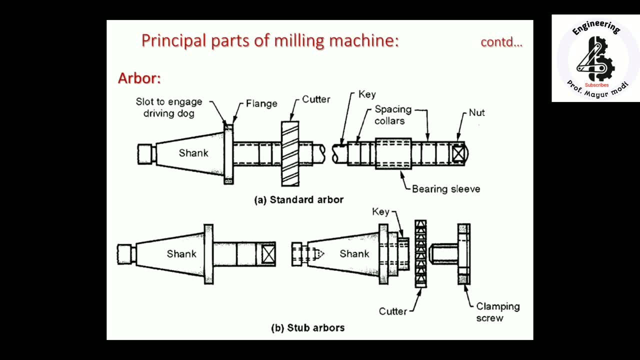 So, according to the my requirements, we are using standard arbors as well as the stub arbors. So For the arbor just, you can see over here in that case of the standard arbors, the slot to engage the driving dock. so that will be the same part with the flange and in the middle 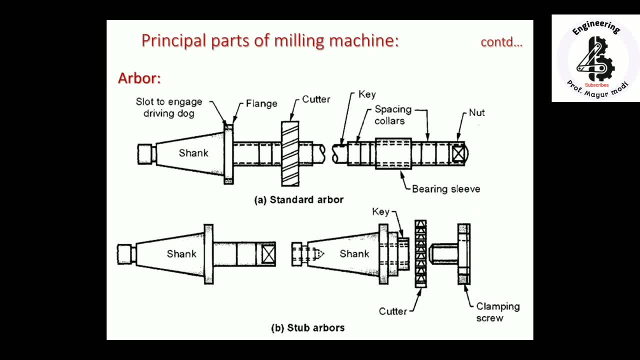 sections- that will be the cutters and spacing collars- is being used for using a number of the milling cutters according to my requirements and that will be all fixed with the help of nut. So just you can see over here that will be the bearing sleeves, spacing collars, keys. 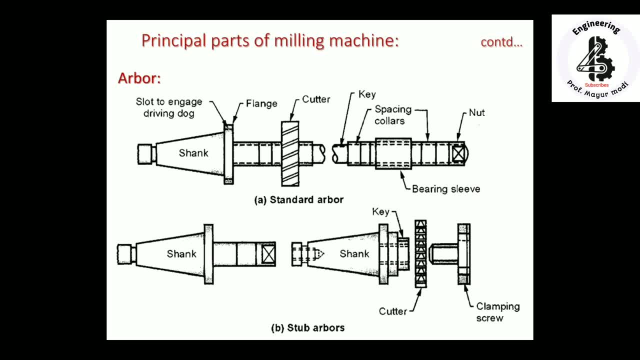 and number of cutters for the standard arbors. Now you can see for the stub arbors over here. so in that case our shank is being fitted with the arbor and in that case that will be the standard type of, or you can say, side.